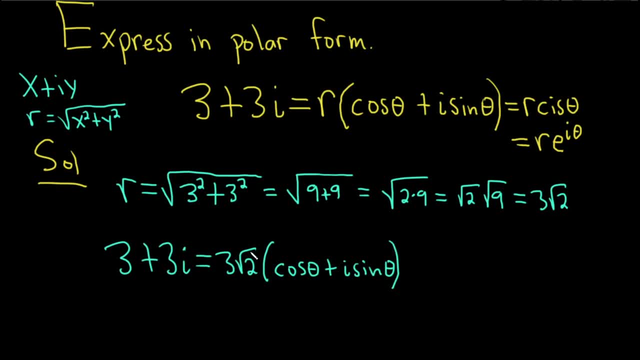 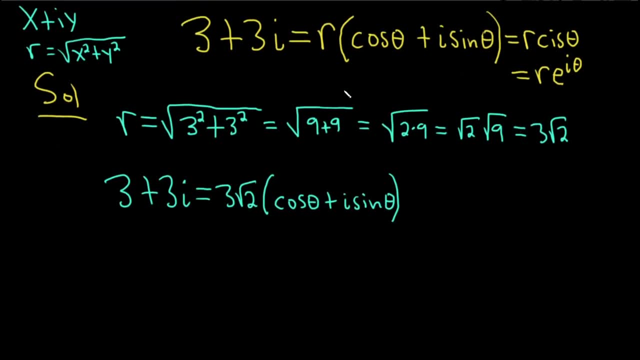 You could do it another way. you can use tangent. I like to do this because it really helps me think about, like you know, the location of the angle and of the complex number. So you find your r, plug it back in And let's get rid of this r by dividing both sides by. So if we divide, 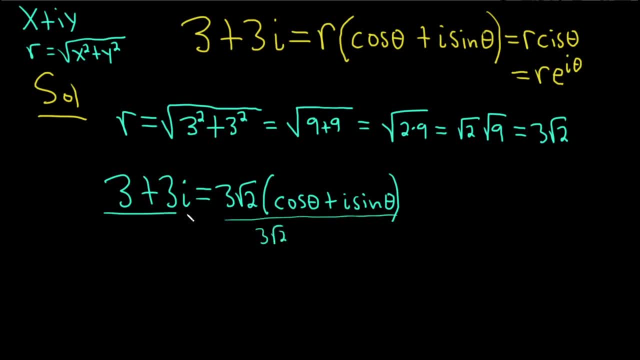 both sides by three root two. we divide each term by three root two, so it'll be one over the square root of two plus one over the square root of two times i. I'm going to write it like that. it's this: over this right, the threes cancel equals cosine theta plus i sine theta. 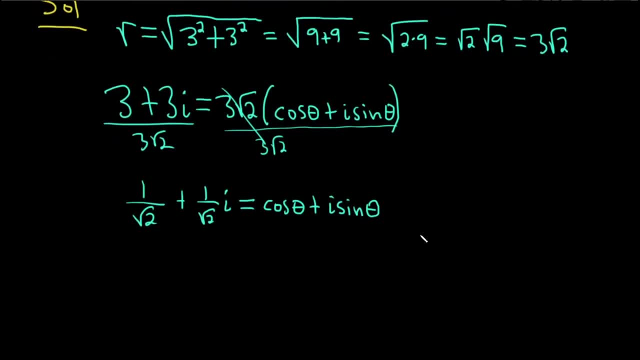 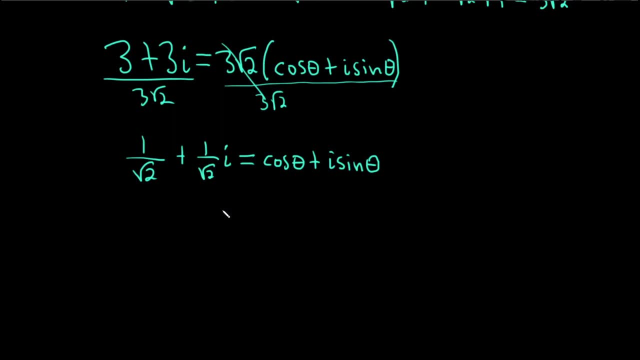 And here's the part I think is cool. So now you can use, you know, the definition of equality for complex numbers, right? two complex numbers are equal only when their real parts and imaginary parts are equal, right? So that would mean that the cosine of theta is equal to this. 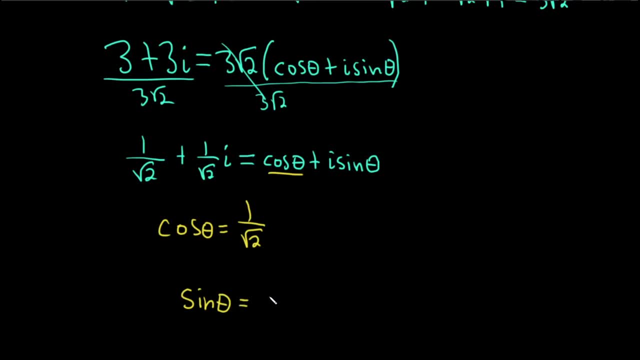 And the sine of theta is equal to this. And if you're not familiar with this, with this fraction, this is really you know. you can multiply this by square root of two over two. square root of two over square root of two. 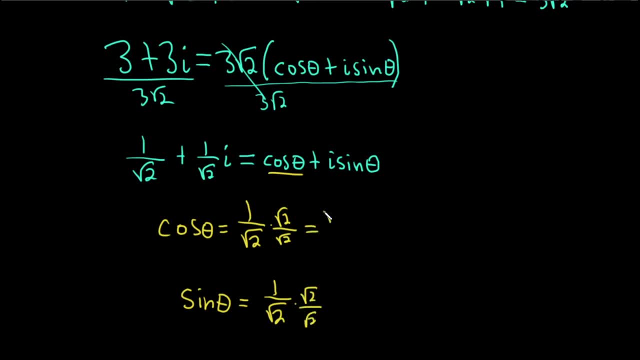 And maybe this will be seen more familiar. this is the square root of two over two. maybe this is how you have it memorized. maybe This is a very familiar angle. it's pi over four, right? So the angle that solves both of these equations, the system of equations. 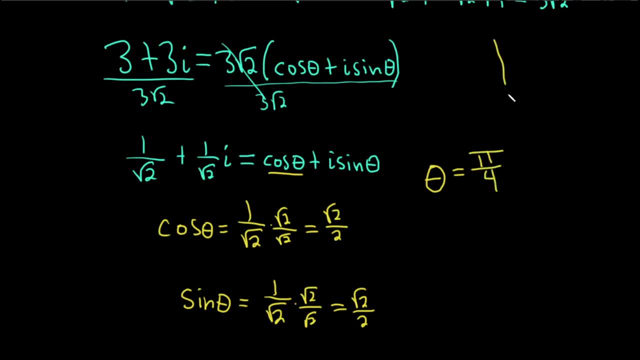 is pi over four. So that's our argument And that makes sense, right? if you look at three plus three, i should be like right here somewhere, right, three plus three i. So, yeah, it looks to me like it's 45 degrees, which is pi over four. So we did it, we've got, we've got it. 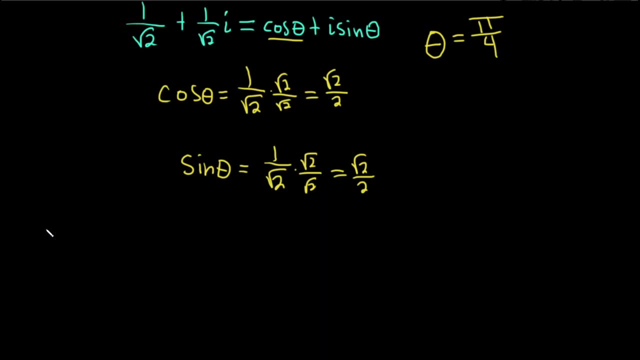 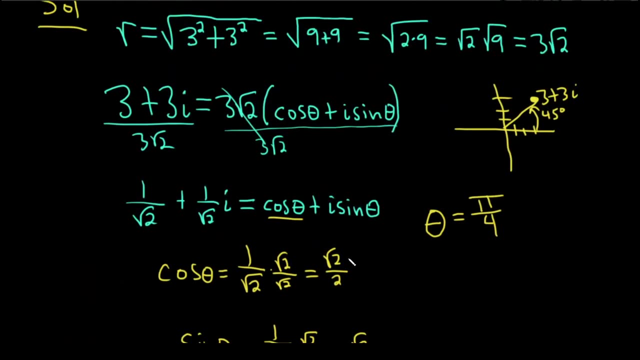 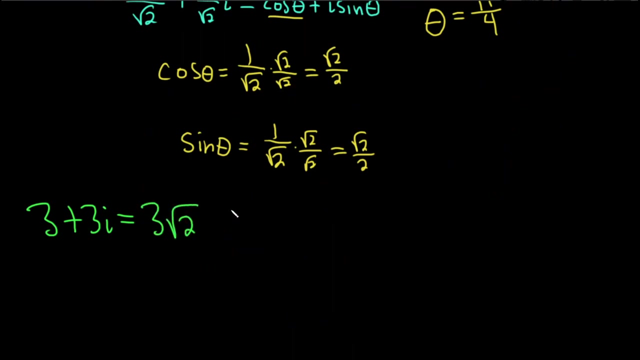 Let's write our final answer down: Good stuff. So this is three plus three. i is equal to r, which I forgot what that was. I don't have this written down. It's three square root of two. This is three square root of two. And then we had parentheses. cosine pi over four. 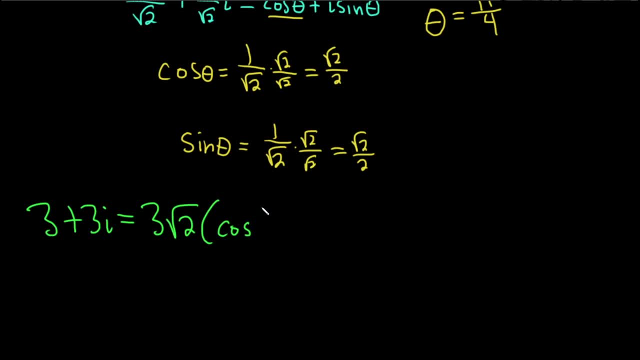 Whoops, whoops, whoops, not theta. theta is pi over four, cosine of pi over four plus i sine pi over four. So this is this is one way to write the answer, right. this would be the polar or trig form.